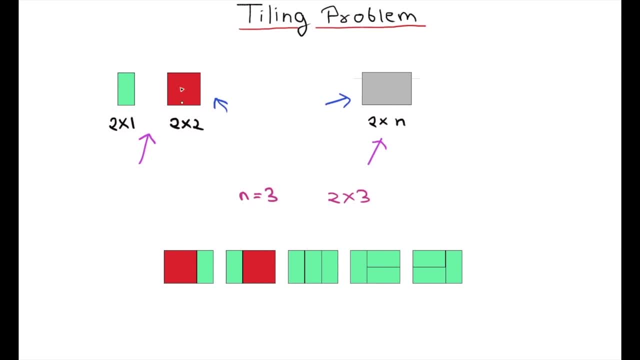 a tile of 2 cross 3 using these two tiles. So there are total five ways to form a tile of 2 cross 3 using these tiles. So let's find how we can solve this problem. Let's suppose this is the space of 2 cross n which we have to fill to. 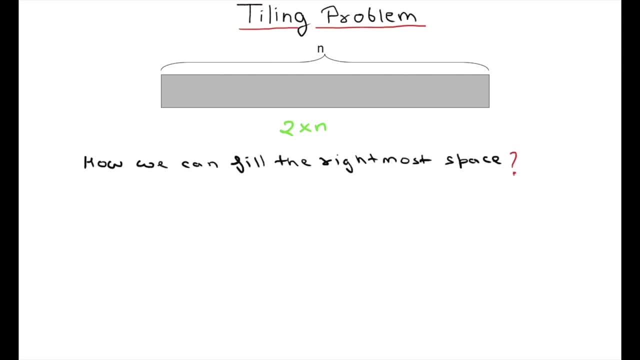 form a tile of 2 cross n size. How we can fill the rightmost space. We can fill the rightmost space by placing a tile of size 2 cross 1 vertically, like this. Second, by using two tiles of size 2 cross 1 horizontally, like this: 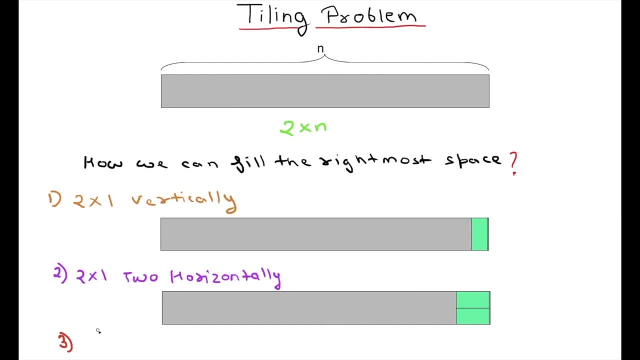 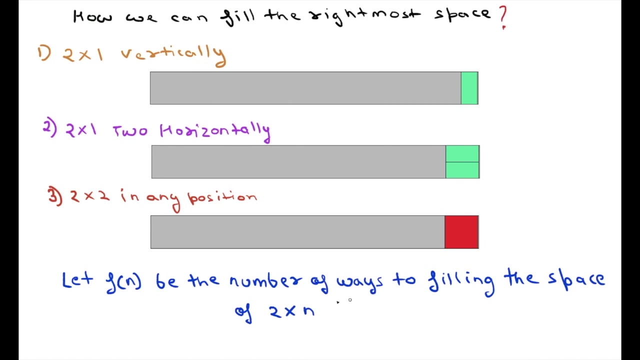 Third, by using a tile of size 2 cross 2, either place it vertically or horizontally, because its size is 2 cross 2, so it remains same in horizontal and vertical position. like this, Let fn be the number of ways to filling the space of 2 cross n. So fn minus 1 will be. 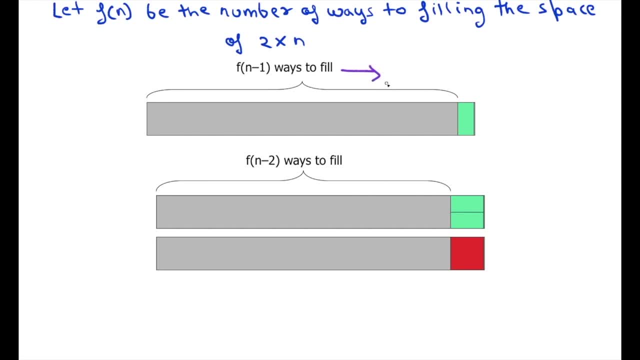 the number of ways to fill the space of size 2 cross n minus 1.. And fn minus 2 will be the number of ways to fill the space of size 2 cross n minus 2.. So the number of ways to fill the space of size 2 cross n, that is, fn, will equal to the sum of the number of ways. 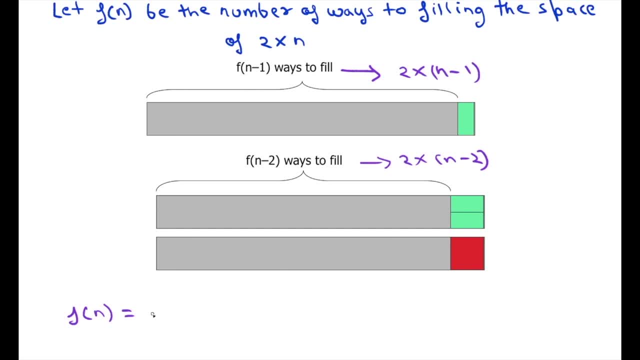 to fill the space of size 2 cross n minus 1, that is f of n minus 1.. 1 plus the number of ways to fill the space of size 2 cross n minus 2, that is F n minus 2. but there are two ways to fill the space of size 2 cross n minus. 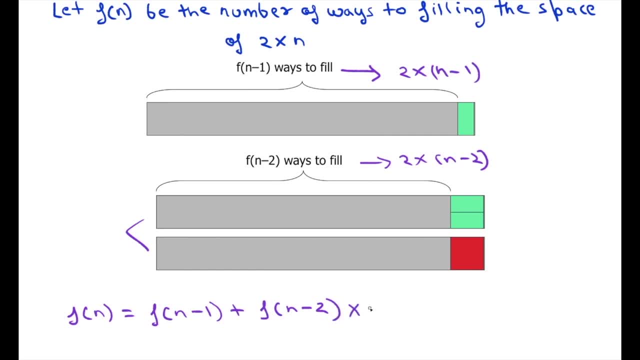 2. so we have to multiply this function with 2. so this is our recursive relation, to find the number of ways to make a tile of size 2 cross n. so this is relation, recursive relation. so we have to find a base case also. so let's find: 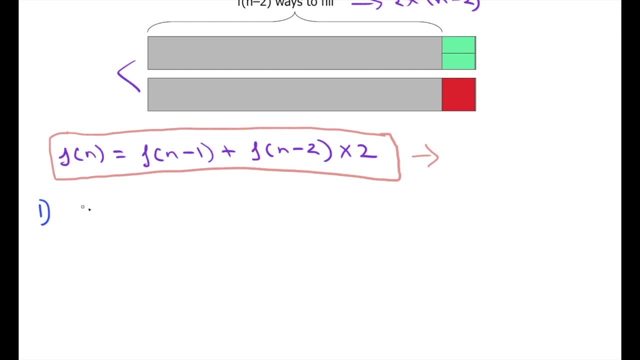 the base cases. the first base case is: F of 0 is 1. but how, if we put, if we put n equal to 1 in this equation, then it will become: F of 1 is equal, F of 0 plus F of minus 1 into 2. 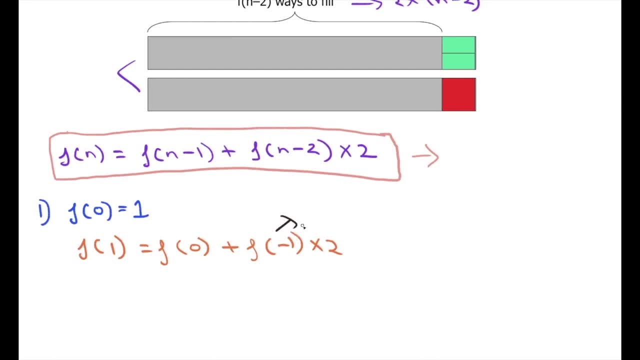 but this is absurd because there is no space of size 2 cross minus 1, so this will become 0 and now our equation will become: F of 1 is equal F of 0. but there is a way to fill this space of size 2 cross 1 by using a tile of size 2 cross. 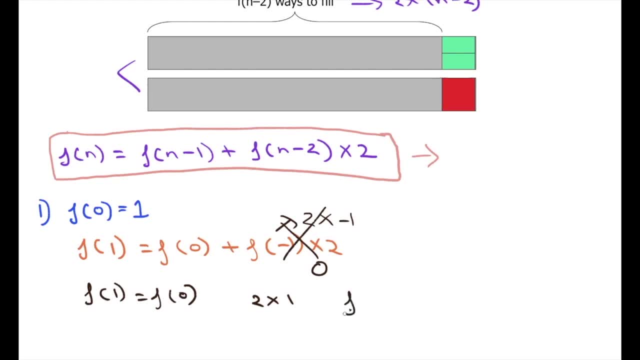 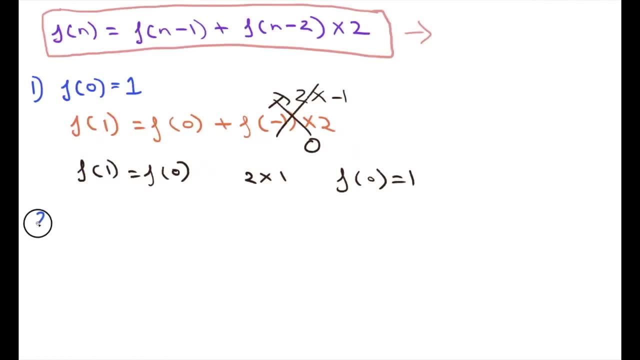 1 vertically must be equal 1. that's why f0 is 1. now our second base case is f of 1 is 1, which is obvious because we have already see here that there is a one way to fill the space of size 2 cross 1: using a tile of size 2 cross 1. so these are our two. 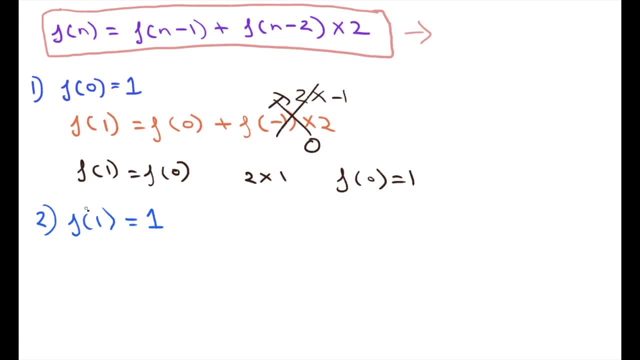 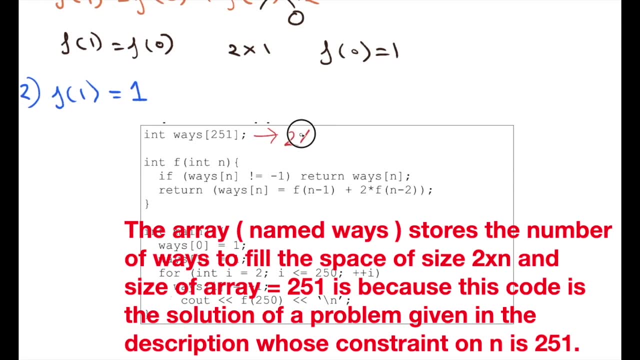 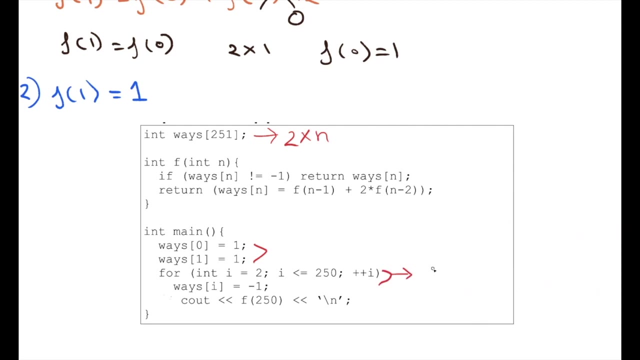 base cases. so let's see the code. the array way stores the number of ways to fill this space of size. 2 cross n, and here we will fill our base cases, and in this line, initially, we fill all our all number of ways with minus 1, that is till. 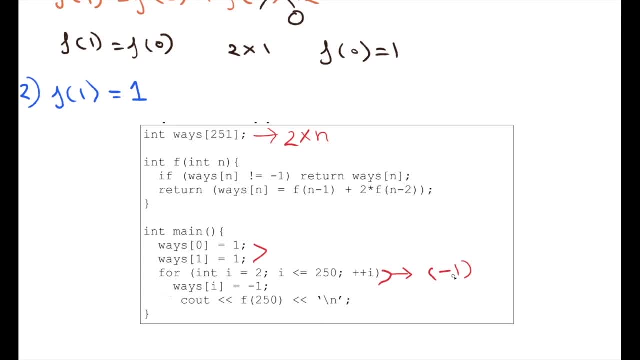 now we haven't compute the number of ways to fill any of the space, and here we call the space of size 2 cross n, and here we call the space of size 2 cross n. Collect all our function to calculate the number of this fill the space of. 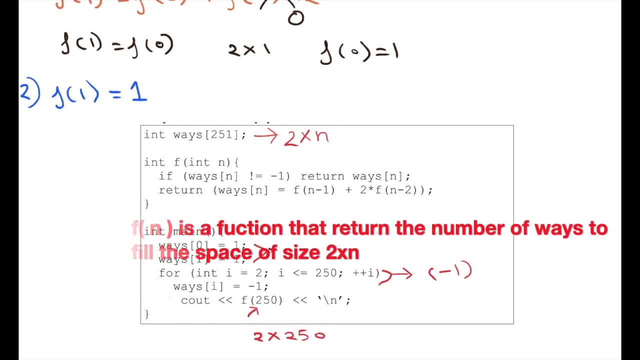 size 2 cross 250. so this is our function, which we call So in this line, if ways of n is not equal minus 1, it means that we have already compute the number of ways to fill this space of current size, and every time we will call our.